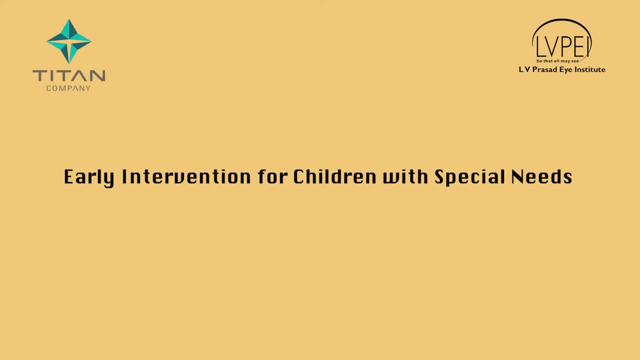 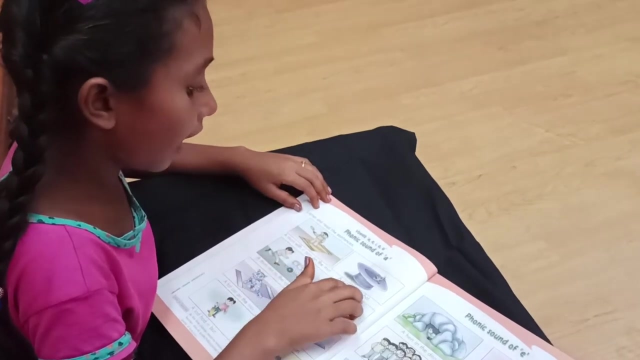 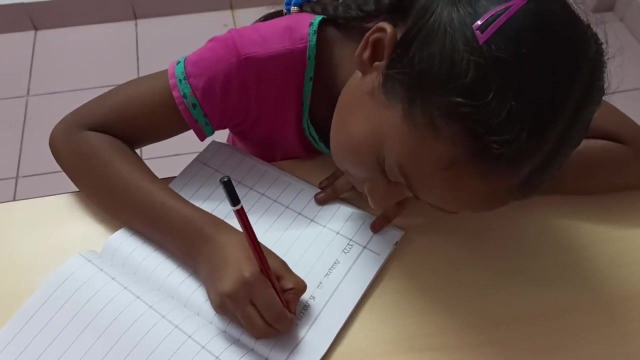 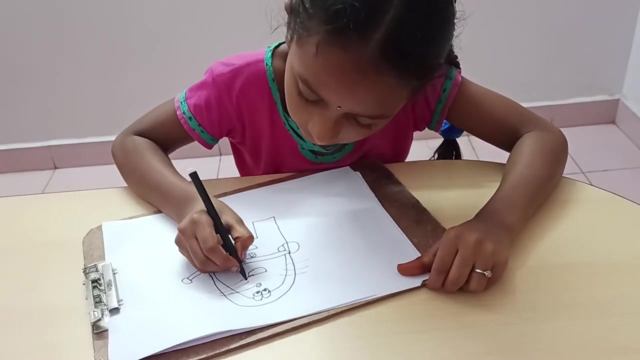 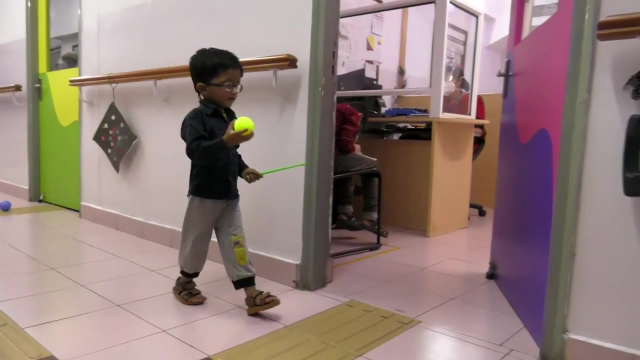 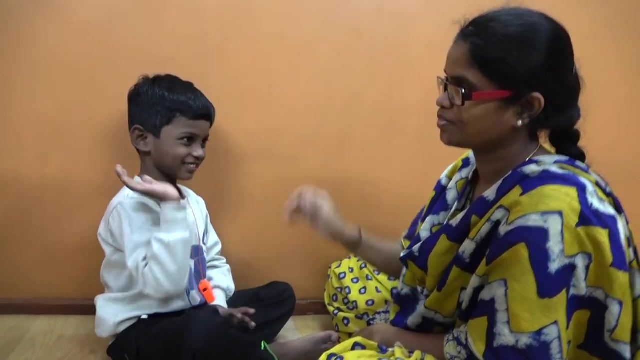 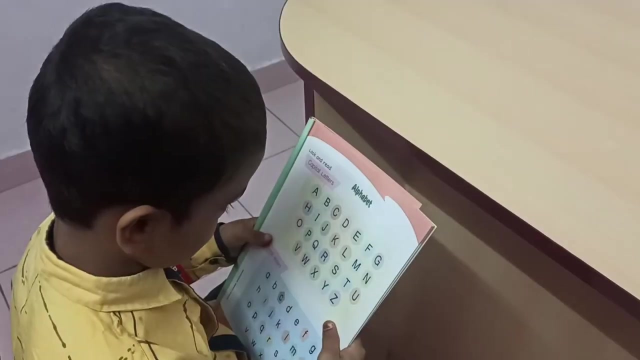 Visual Perception is the ability to interpret the visual information, which is important for daily activities such as reading, writing, drawing, drawing, drawing drawing drawing drawing drawing, Playing and moving from one place to another. In children, visual perceptual skills are important to improve their self-esteem, academic performance and participation in daily activities. 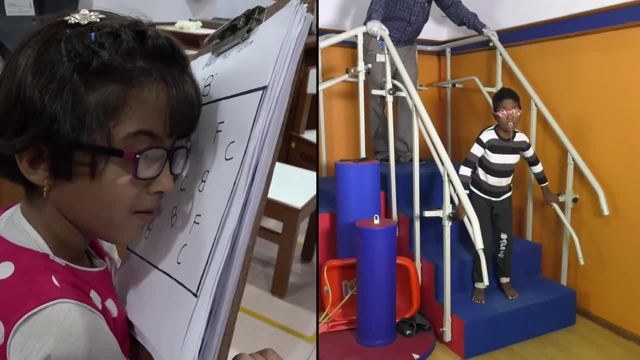 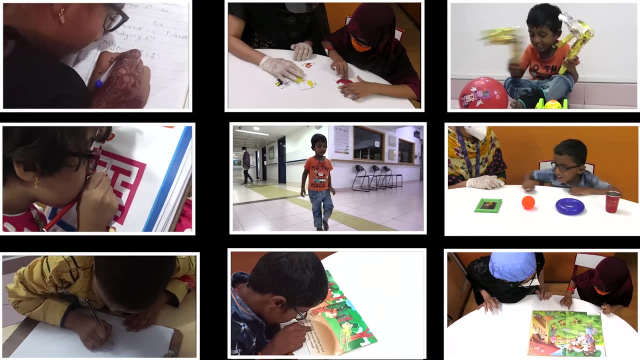 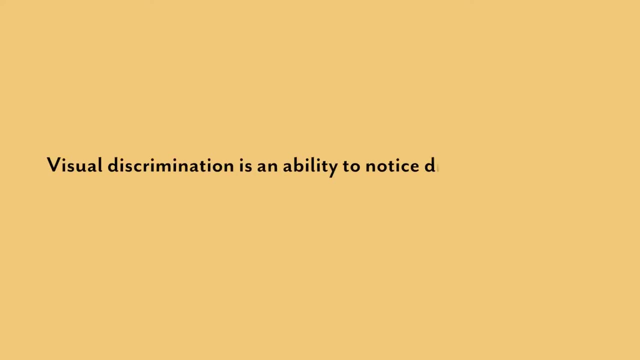 Children with impaired vision may have problem in visual perceptual skills. These videos are exclusively developed with the aim of improving various visual perceptual skills in children with visual impairment. Visual Discrimination: Visual discrimination is an ability to notice difference between one object to another by its color, form, place or size. 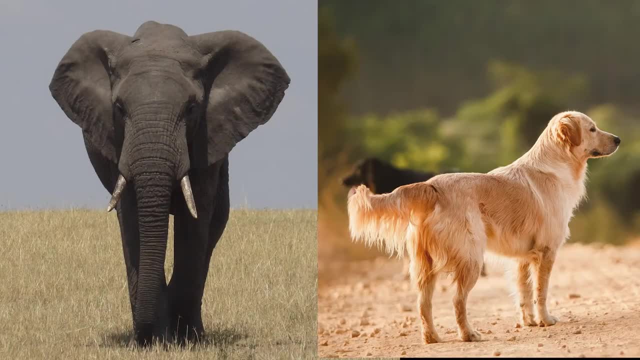 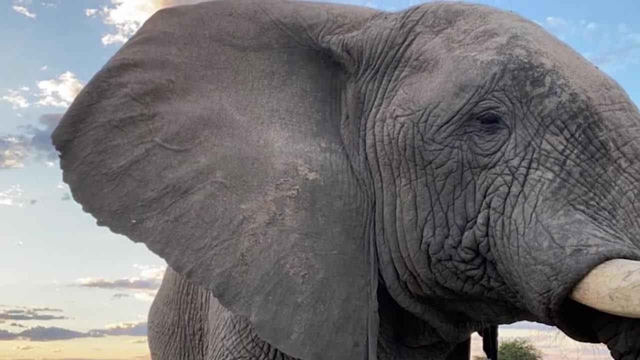 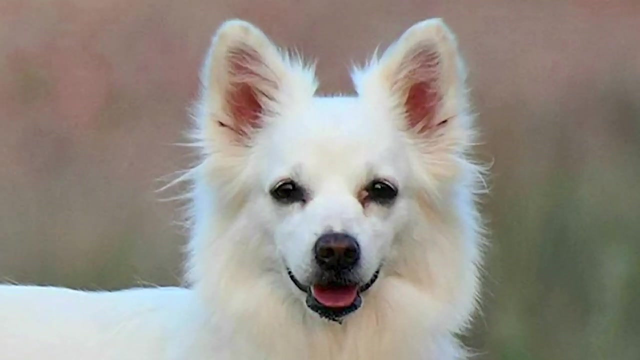 For example, discriminating between an elephant and a dog. An elephant is big in size, Has a trunk, Is grey in color, Has thick skin and big ears. In comparison, dog is small in size, varies in color, has silky fur and has small ears. 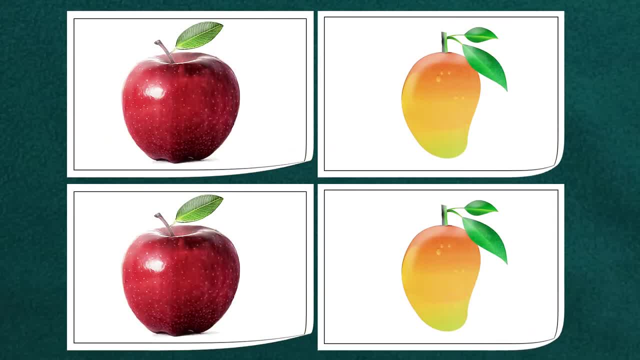 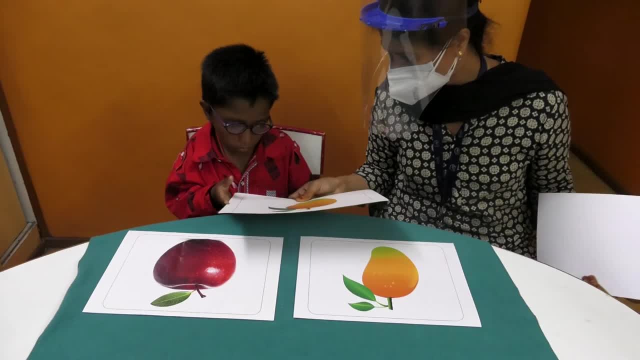 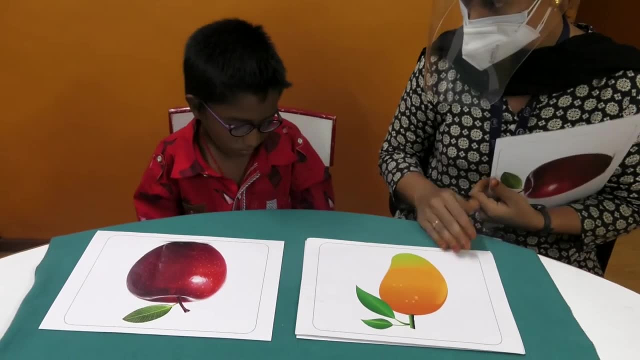 Activities to improve visual discrimination. Take two sets of matching cards. Display one set of card on the table and give a single card from the second set to the child. Now ask the child to match it with the same picture. This activity will help the child to develop discrimination. 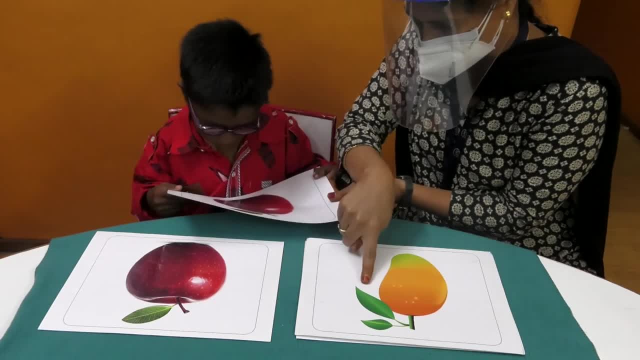 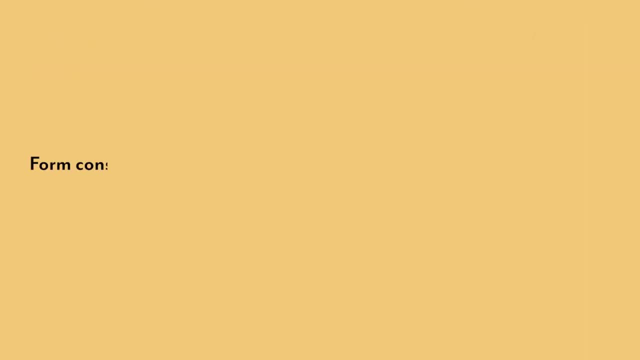 This activity will help the child to develop discrimination skills by discarding all other cards which are not the same. Form Constancy: Form Constancy is the ability to identify objects even if they are different in sizes, places, positions and shapes. activities to improve the skill of form constancy. 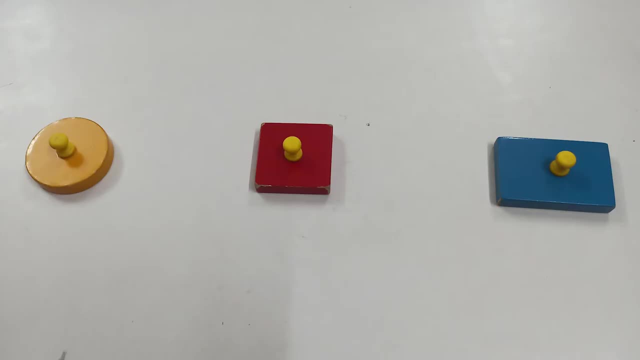 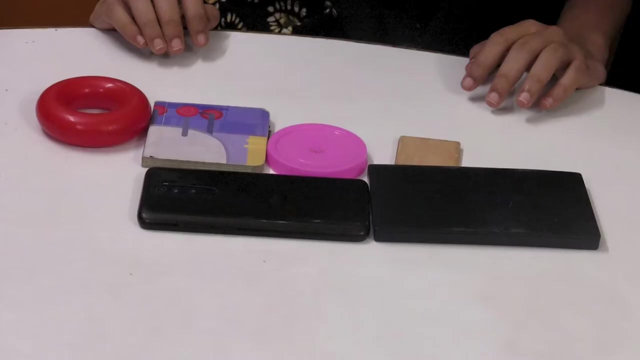 Shape Constancy On a table. keep wooden blocks in the shapes of circles, squares and squares. Keep wooden blocks in the shapes of circles, squares and squares, squares and rectangles. now give objects that are similar in shapes to the wooden blocks to the child. 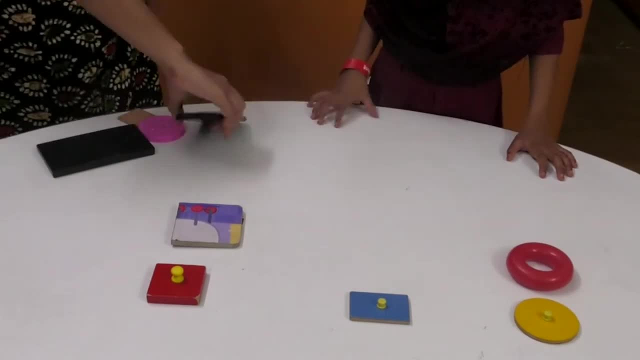 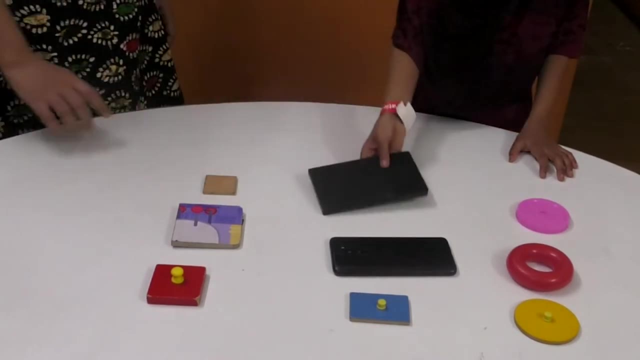 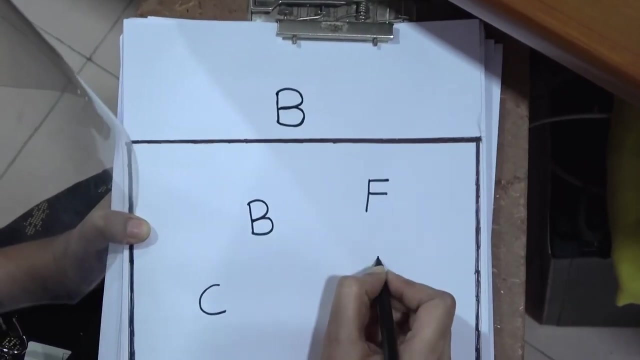 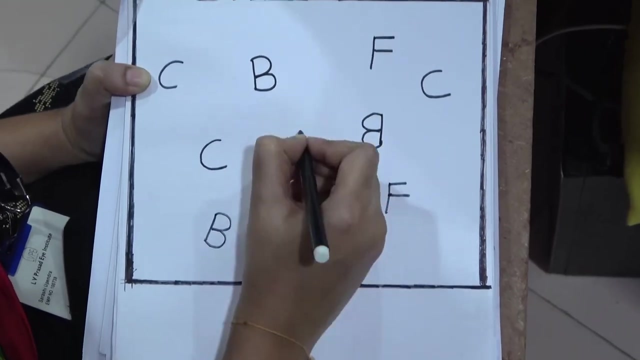 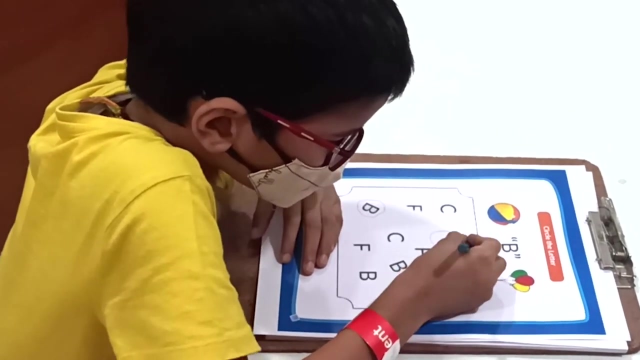 and ask the child to match them with the wooden blocks by their shape, position, constancy. write a few random alphabets on paper. select a particular alphabet, like say b. write it multiple times on different positions. now encourage the child to identify and circle all the bees written in different positions. 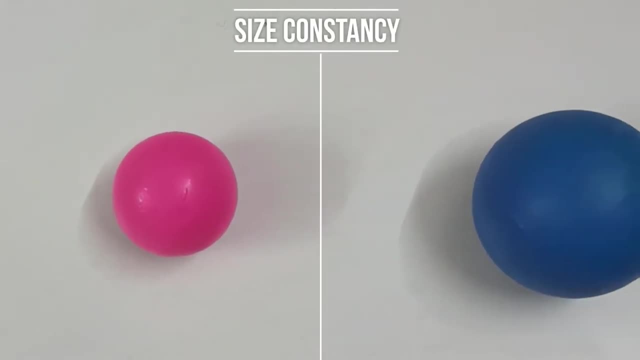 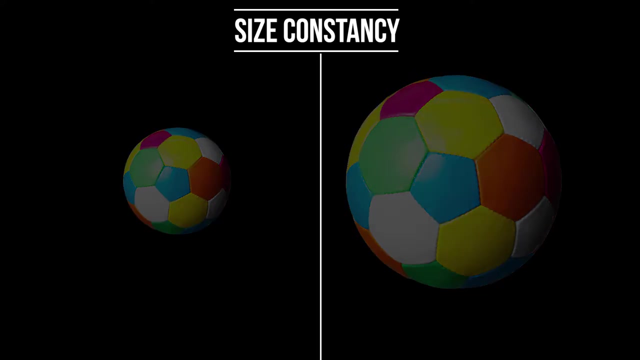 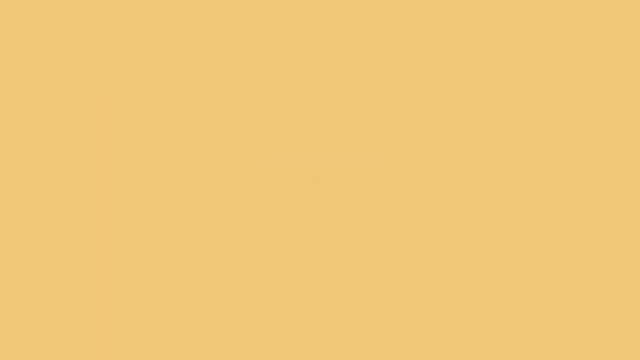 size constancy. to introduce size constancy to a child, take objects of the same properties but of different sizes. example balls of different sizes from small to big, or water bottles from small size to large size to big size. Visual closure: Visual closure is the ability to recognize. 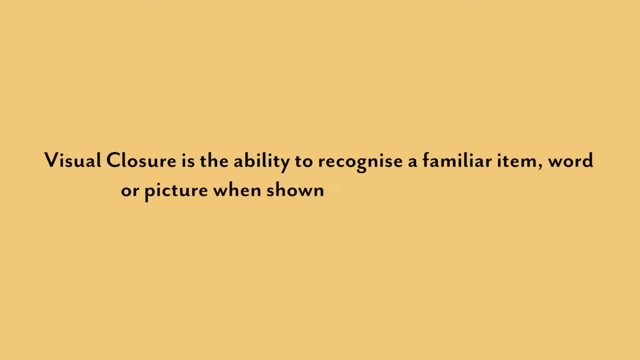 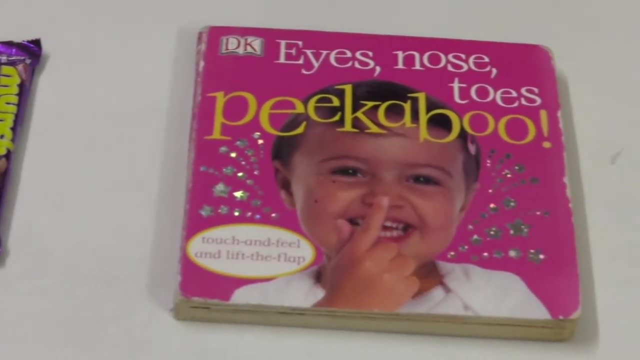 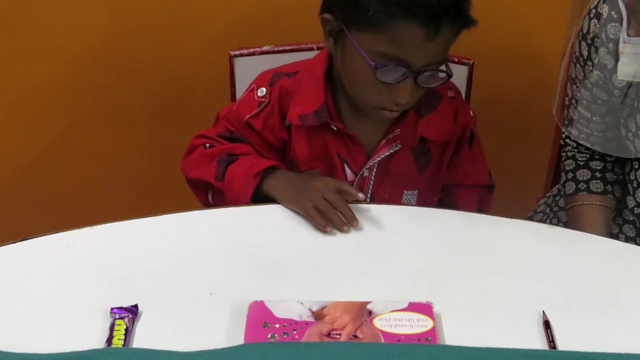 a familiar item, word or picture when shown only a small part of it. Activities to improve visual closure. Take some items that are familiar to the child and place them on a table, Partly cover the items with a cloth and ask the child to recognize them. 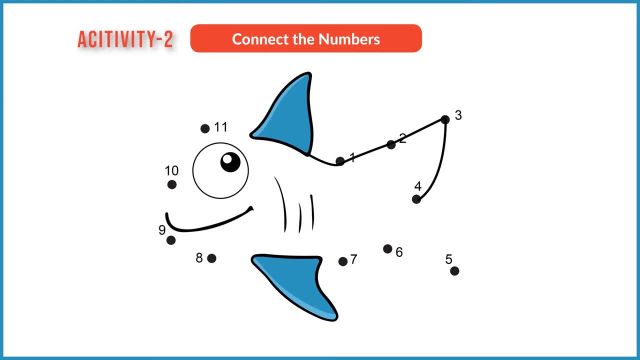 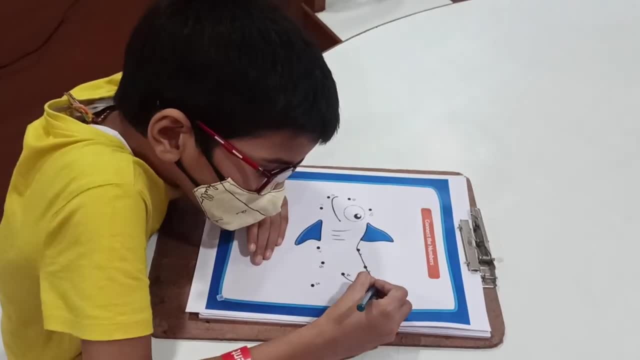 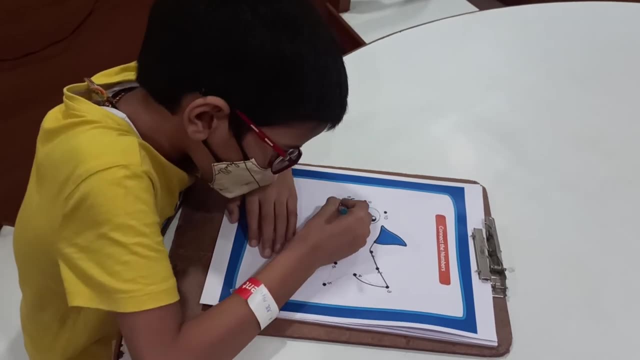 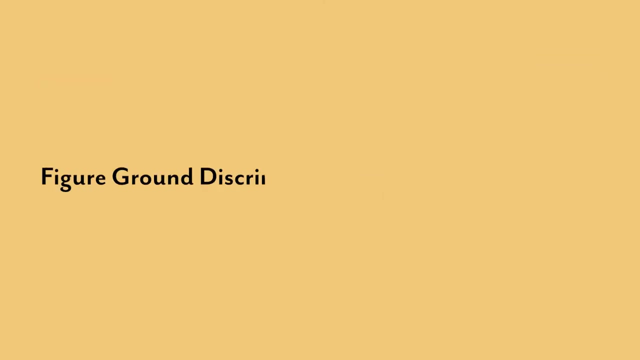 Visual activity. Ask the child to identify the picture For easy recognition. in younger children, in addition to the salient features, they may be asked to connect the numbered dots to make out the shape. Figure ground discrimination. Figure ground discrimination is the ability to identify an object from a busy background. 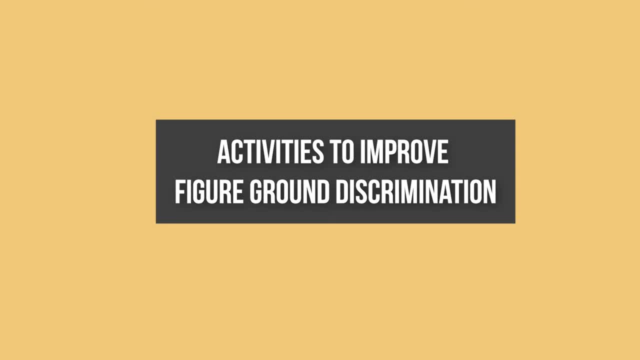 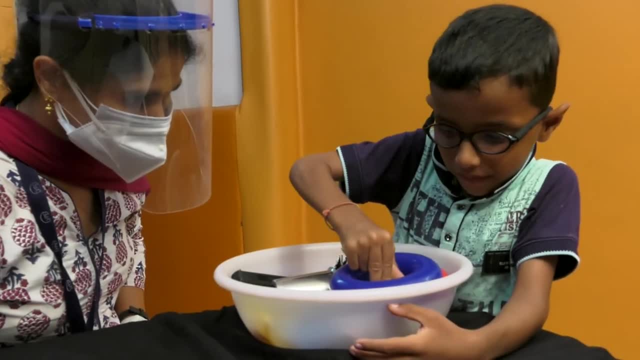 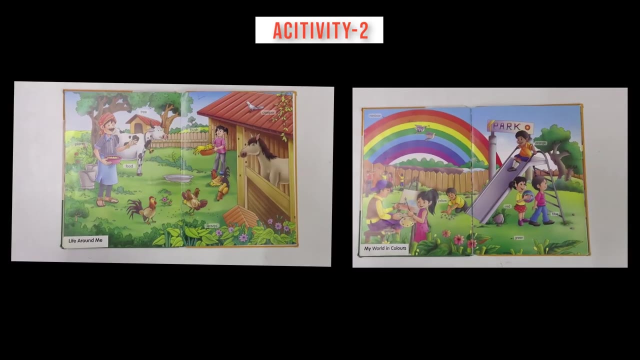 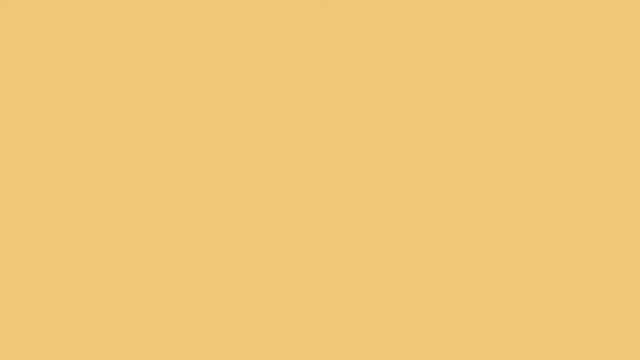 Activities to improve the skill of figure ground discrimination. Keep a variety of objects that are familiar to the child in a basket. Ask the child to pick a particular object from the pool of objects. Another activity: Ask the child to search and find a specific picture from the group of pictures. 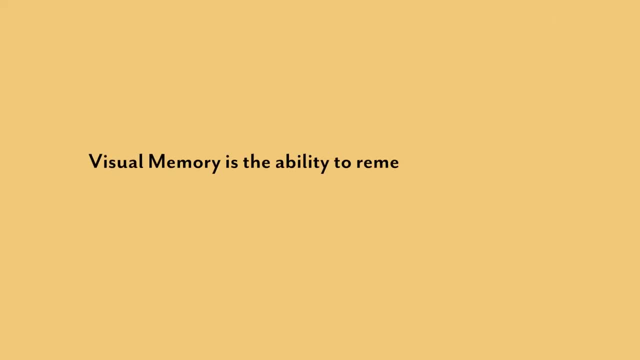 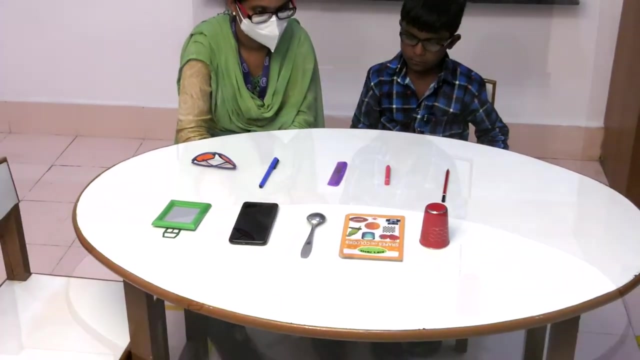 Visual memory. Visual memory is the ability to remember information obtained by visual experience. Activities to improve visual memory: Play memory games to improve visual memory. Keep a few items that are familiar to the child on a table. Ask the child to have a close look at all the items. 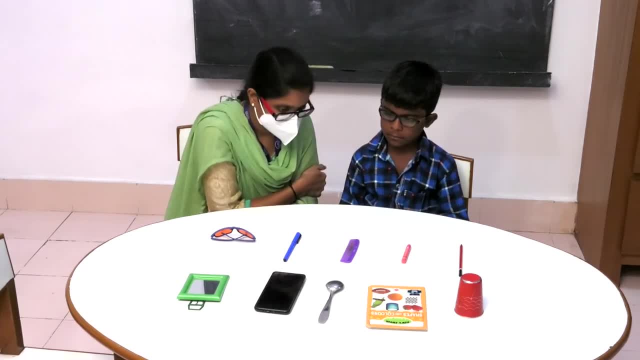 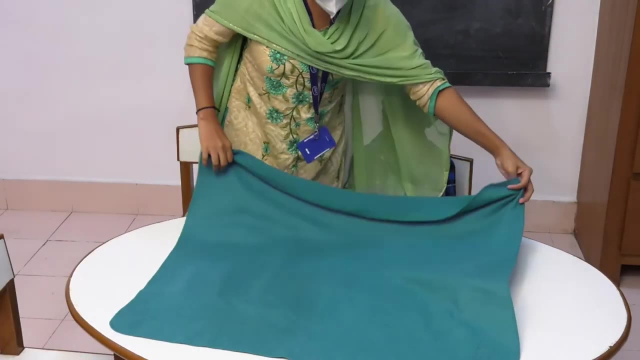 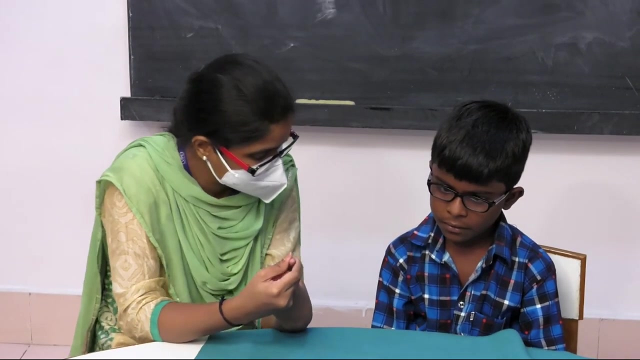 Now encourage the child to understand their properties and memorize the displayed items. After some time, cover all the items with a cloth and ask the child to recollect information of the seen items, such as their names, colors and sizes, etc. 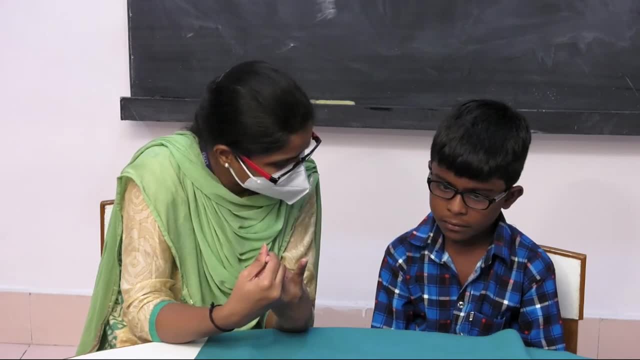 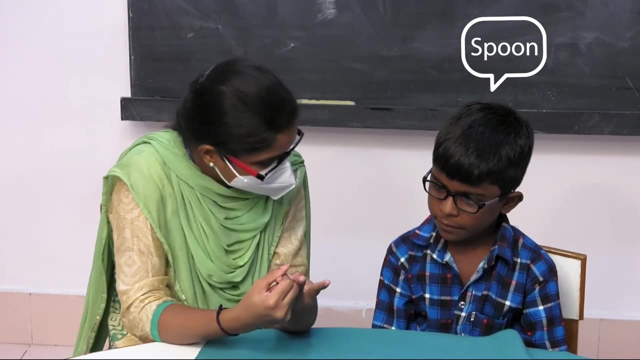 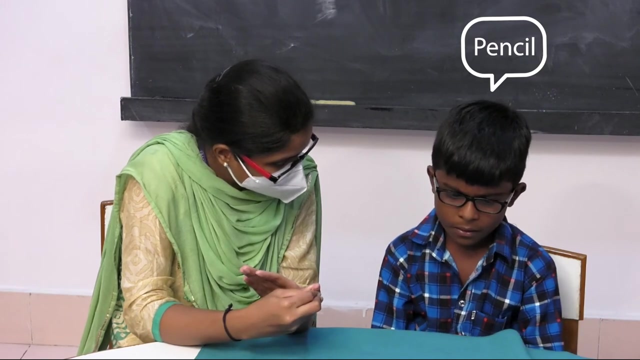 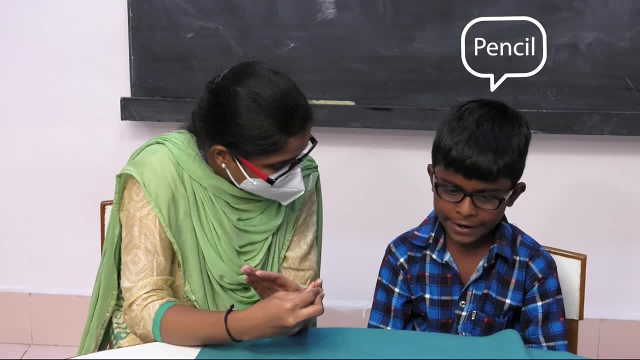 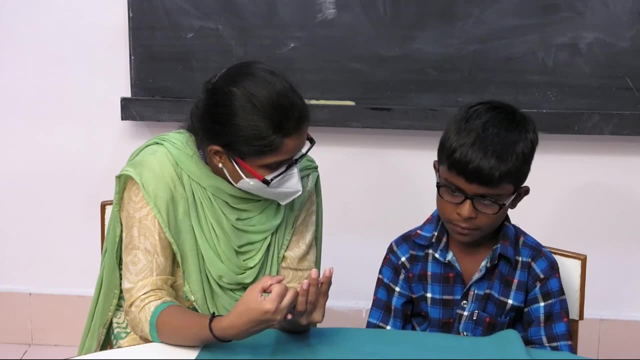 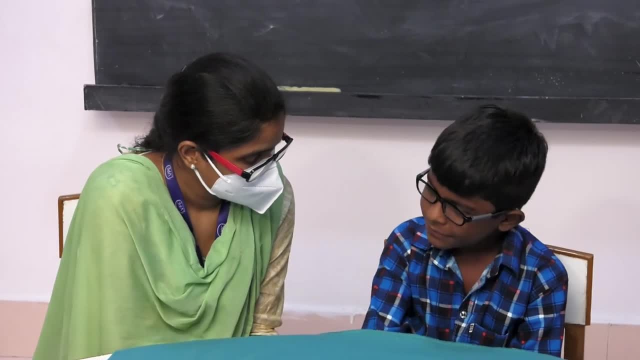 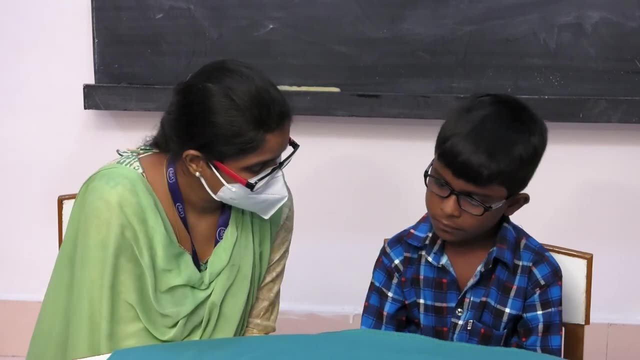 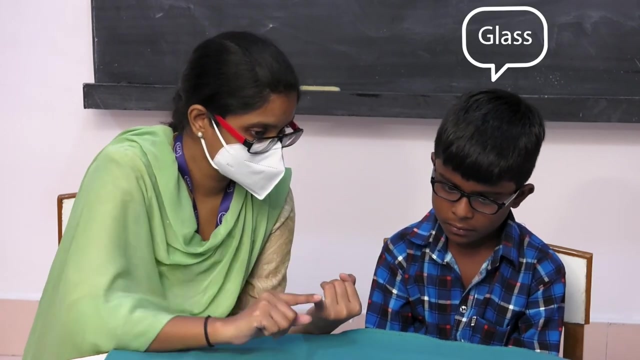 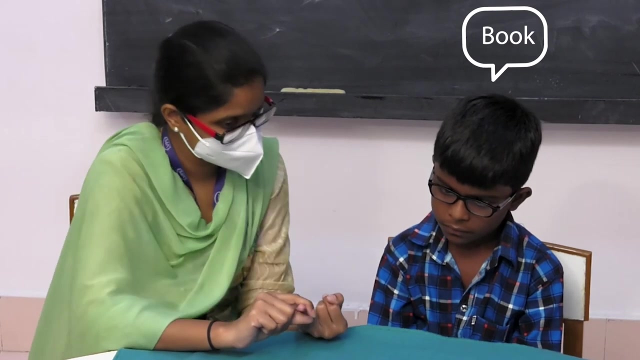 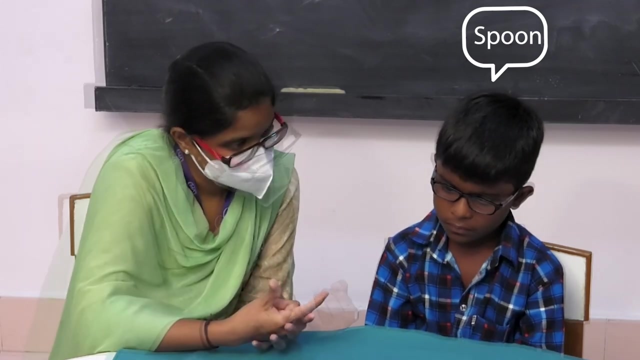 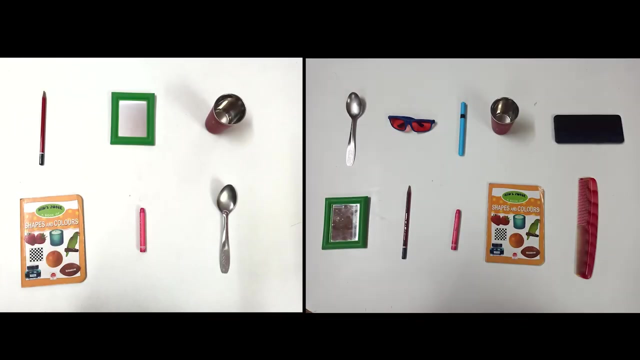 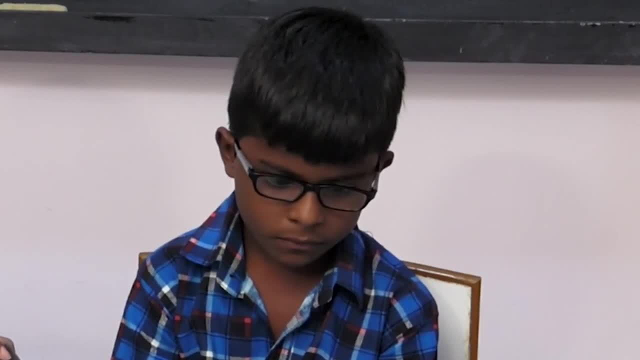 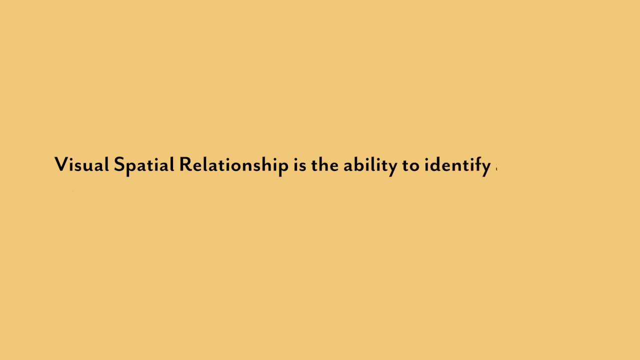 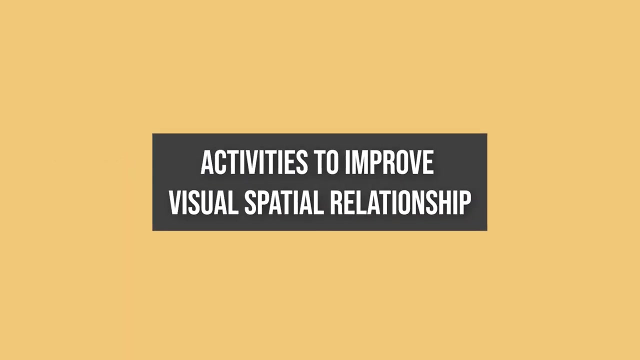 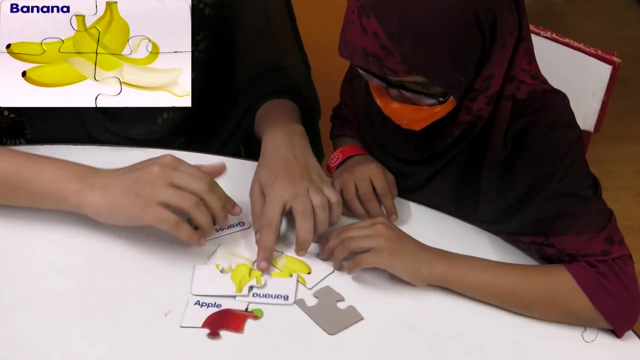 the information based on the child's performance. Visual Spatial Relationship: Visual Spatial Relationship is the ability to identify an object's physical position and visually perceive spatial relationship. activities to improve visual-spatial relationship: Introduce a picture puzzle to the child. Now ask the child to fit the pieces of the puzzle. 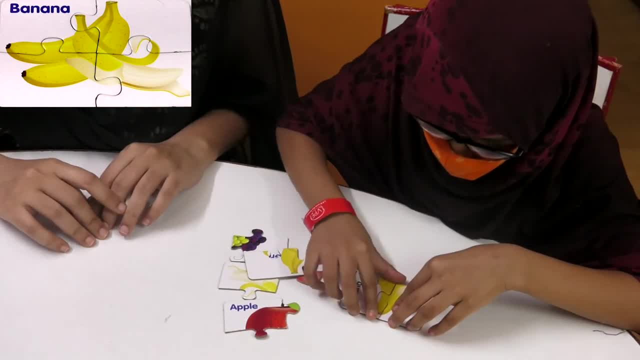 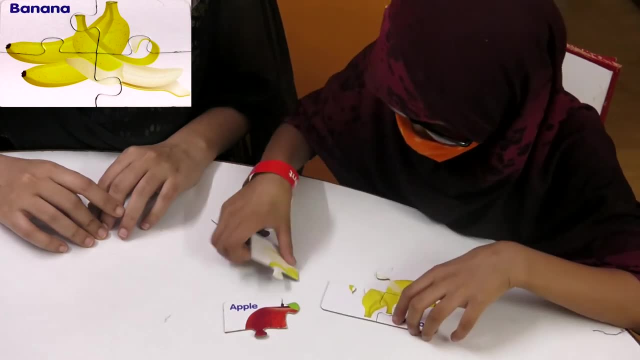 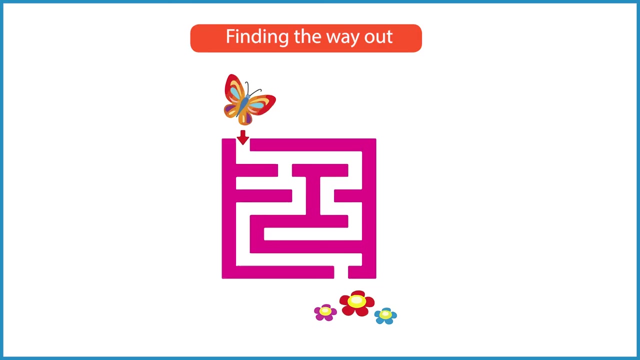 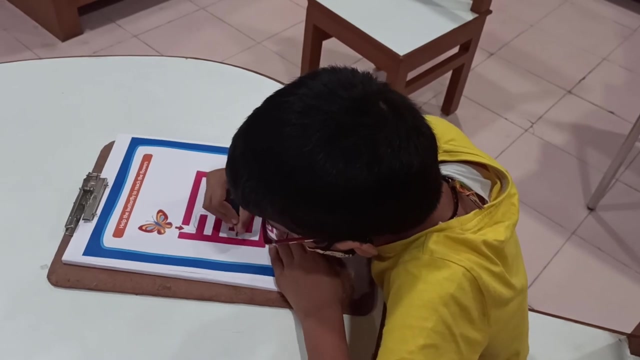 Encourage the child to connect the different pieces. Now ask the child to fit the different pieces to form the image. Another activity: Finding the Way Out. Encourage paper games such as Finding the Way Out where the child is expected to explore the road map to finish the game.